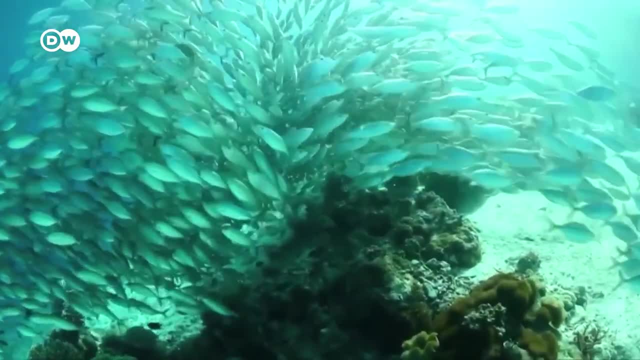 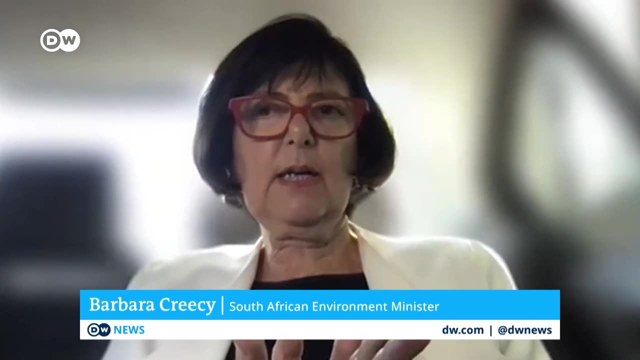 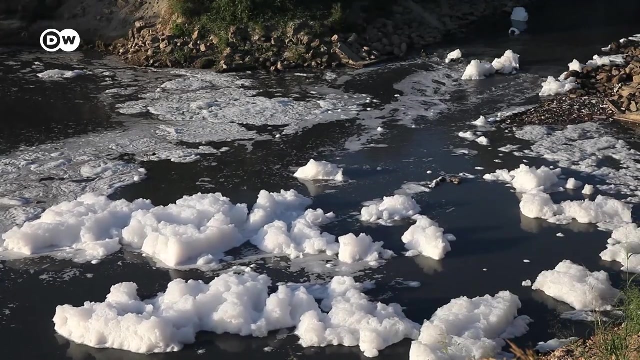 But these countries argue that they lack the resources to expand their conservation efforts. They are demanding financial support from richer nations. We don't want to see a target which has absolutely no hope of implementation. Scientists say there is no time to lose. However, even if the COP15 participants set an ambitious target, it can only be the beginning. 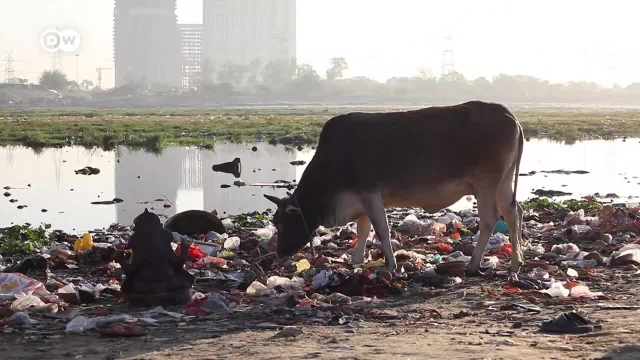 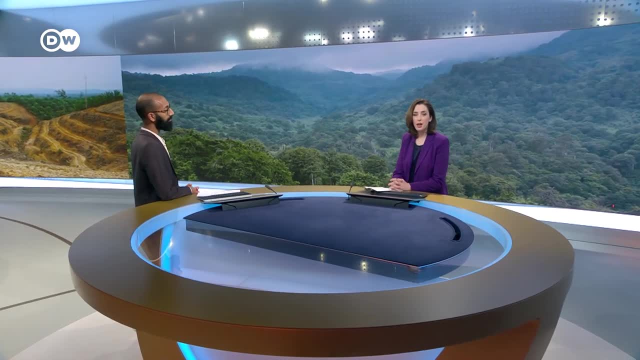 None of the biodiversity objectives agreed at the 2010 convention have yet been fully implemented by the global community. Ajit Narayanan joins us now from our environment desk. He's been following this for us. There's so much at stake at this conference. 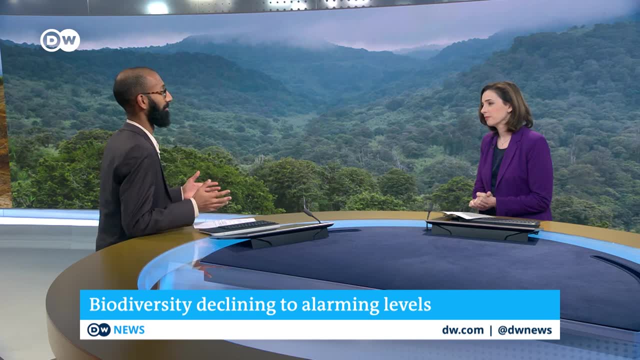 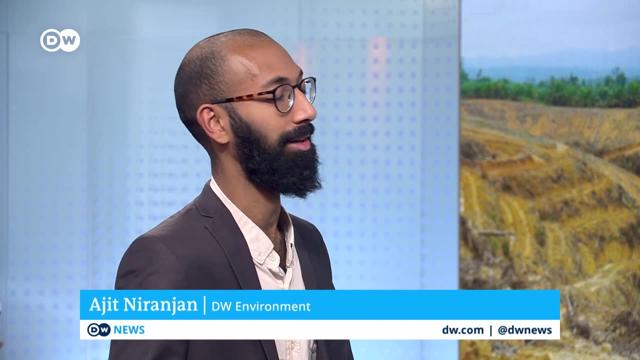 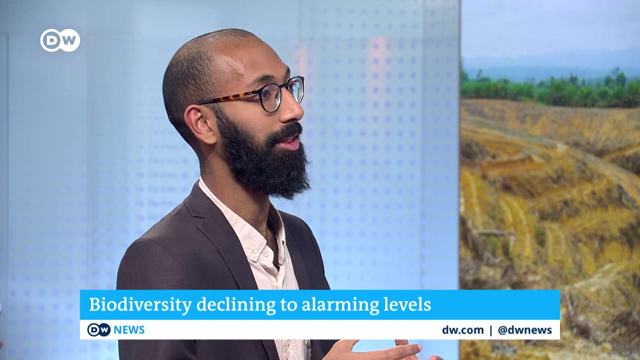 Just walk us through what it is. So, ultimately, this conference is about stopping the destruction of the planet, of the life on this planet, And, as we just heard in the report, we're a long way off actually achieving those goals. So I mean just to give a bit of context. the biggest scientific study of all the life on Earth found just a few years ago that nature is declining at unprecedented rates. 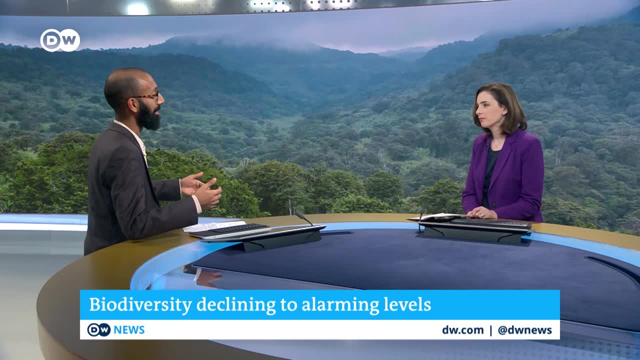 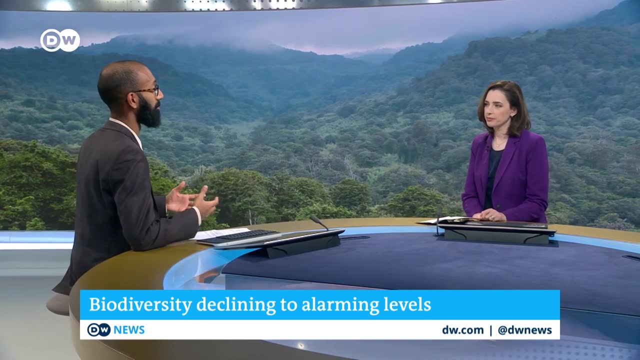 And the rates at which we're pushing species to extinction is getting faster and faster and faster, And so the sort of things that this conference, the parties at this conference, are trying to agree on are policies to do things like protecting 30% of the land and sea from human interference. 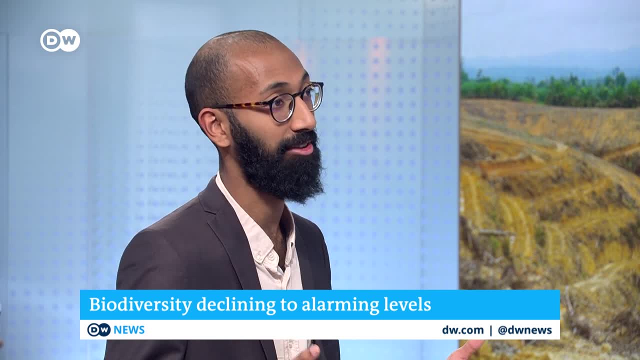 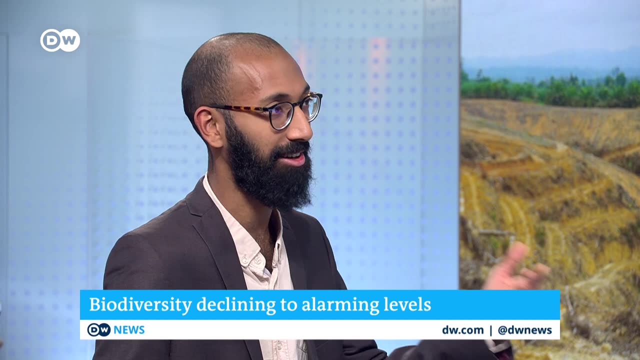 doing things about the huge amounts of fossil fuel subsidies and other environmentally destructive subsidies that essentially taxpayers are using. governments are using taxpayer money to put into the destruction of the things that we rely on, And other policies include things like forcing big companies to disclose, kind of 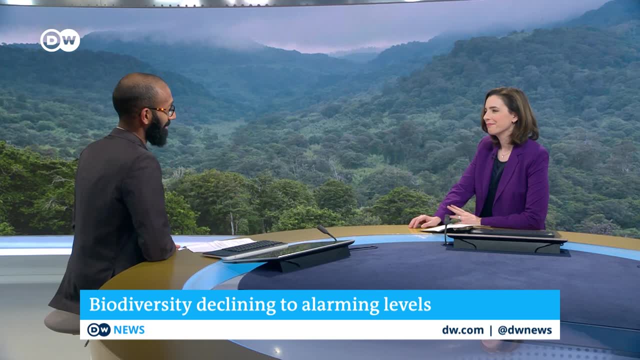 the impact that they're having on nature. Why should we care? It's a good question And it's one that I think scientists. when I talk to scientists about this, I also struggle to get a very clear answer. I mean, there's three ways I think you can look at it. 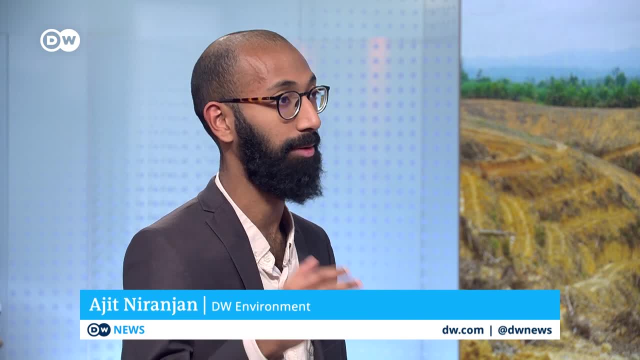 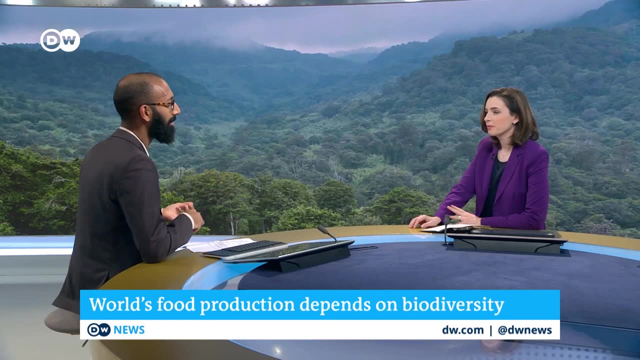 On the very first level is that we pay for it. So we pay for it today in terms of things like when pollinators die and food prices rise and crops die, Bees going, birds going- All of these things mean that we're actually directly suffering from the added costs that we don't see. we don't directly notice it.